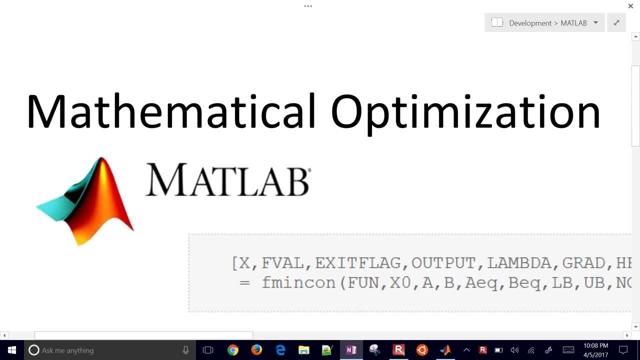 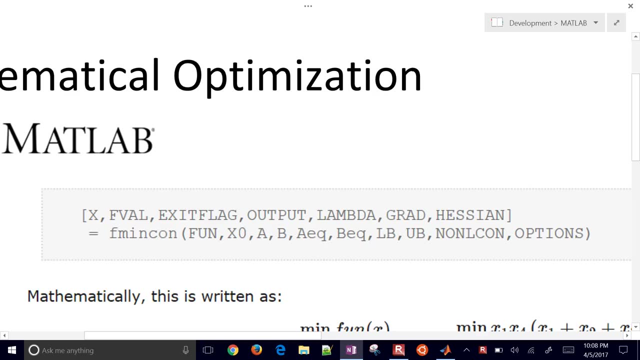 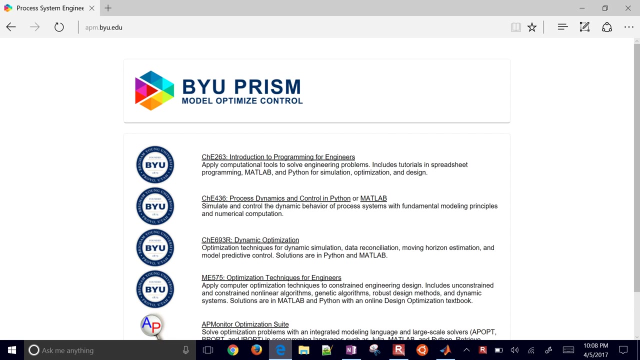 We're going to cover mathematical optimization with MATLAB. In particular, we're going to use this function, fmincon, to solve a nonlinear optimization problem. Now, if you go to the documentation for fmincon, you're going to feel a little bit overwhelmed by all the options. So we're going to just solve a minimal problem here. And if you go to apmonitorcom, you can select, take a course. This material is listed under the intro to programming And if you go down on the 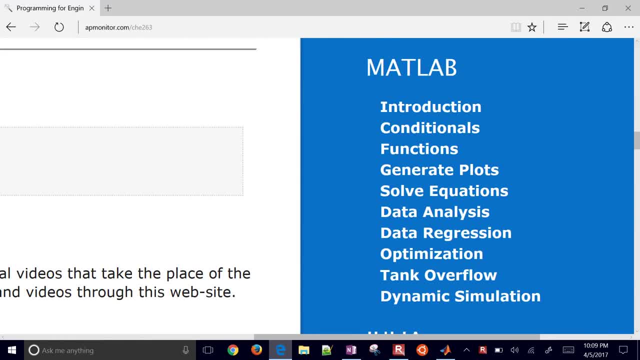 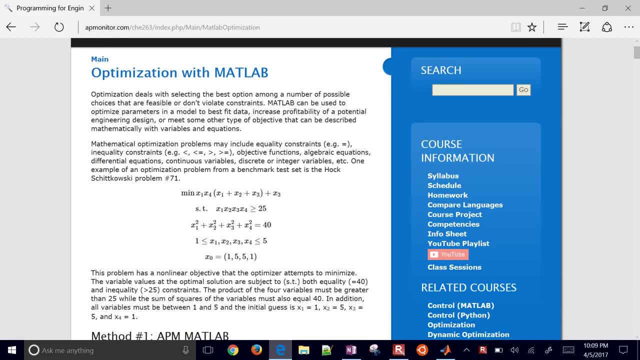 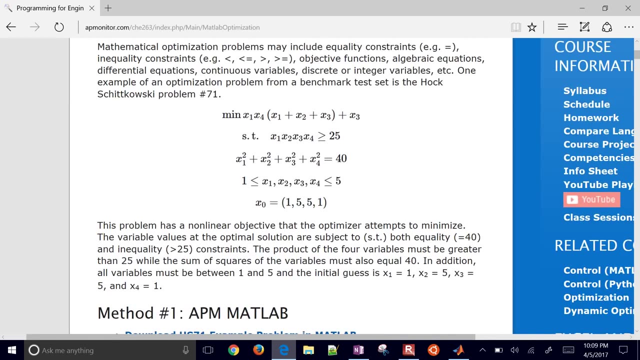 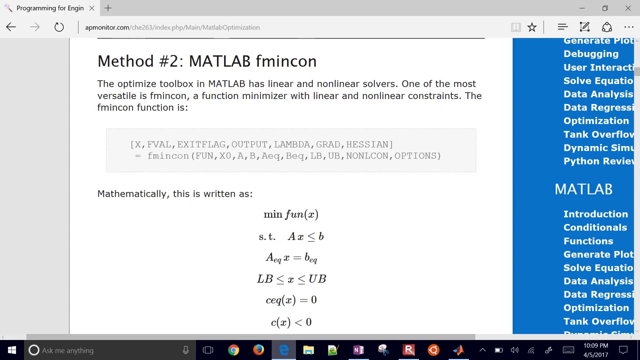 right, you're going to go down to MATLAB and then just select optimization there. Now this shows the problem that we're going to solve. It just has one inequality constraint, one equality constraint, some bounds on the variables, just four different variables there. Okay, the first way that we can solve this is with APM MATLAB. There's a video there if you want to go look at that. This one's the MATLAB fmincon tutorial And it shows how to set it up and solve it with the example source code. 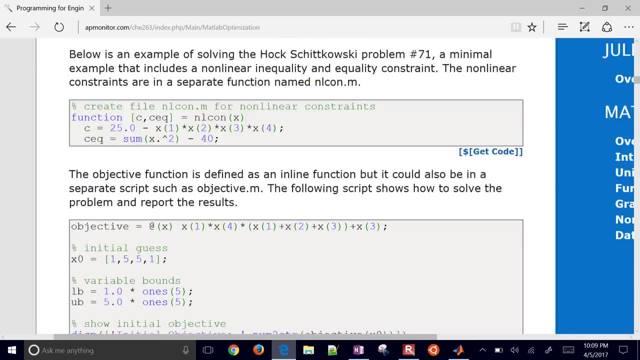 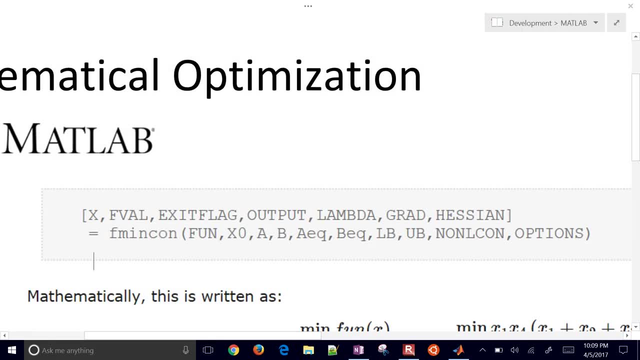 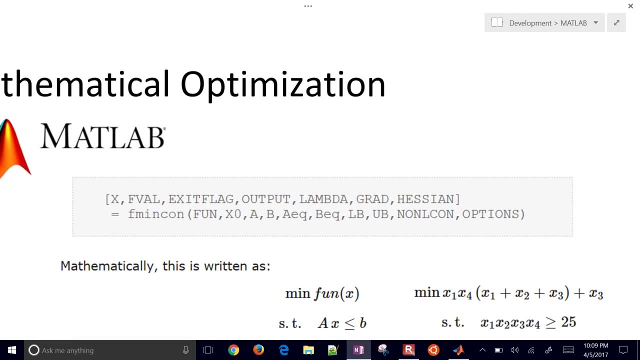 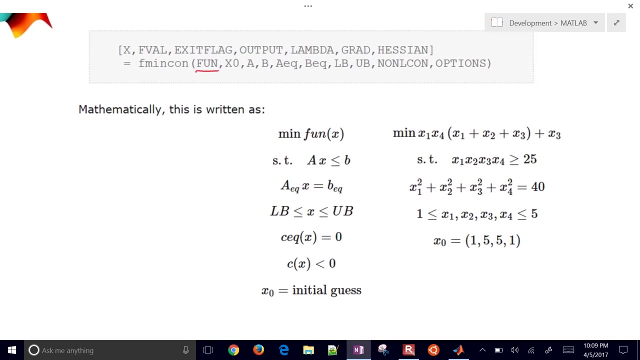 You just select the get code on the right, you can go and download that example. So if you just want to skip to that and go grab the code, you can do that. We're going to work through it in just a little bit more detail and explain it as we go through. So here's the function. right here You have a number of things that you want to input to this function. There's your objective function right there, the FUN. Okay, I'm going to scroll down a little bit. So just as I talk about this, you're going to minimize- we always minimize- the objective function. you can change that. 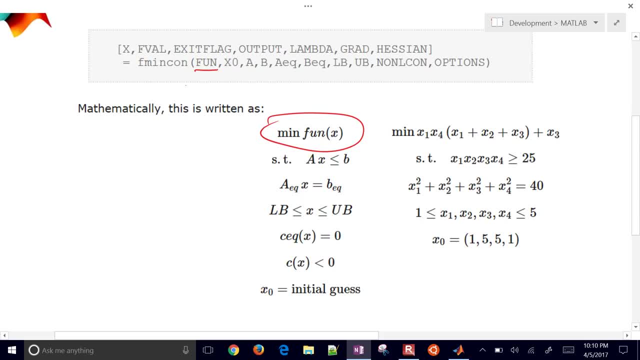 option to maximize, or you can just take a maximization, multiply it by negative one, it becomes minimization. Okay, you want to give it the initial guesses as well. Now, this specific problem: those initial guesses are just one, five, five and one, those are four values. Okay, we also have our A and B right there, those kind of go together. those are our inequality constraints right there for the linear inequality constraints. So A and B are going to be matrices or vectors, And 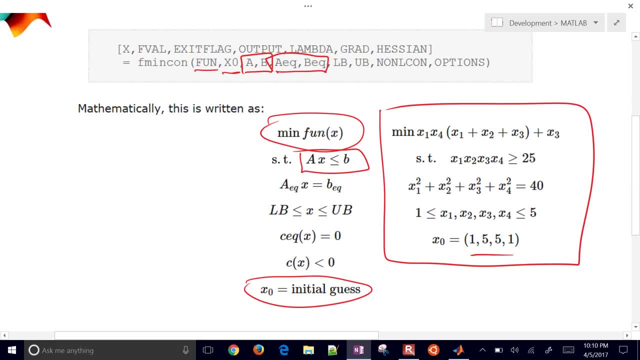 then also Aq and Beq. those are equality constraints. Okay, again, those are linear equality and linear inequality constraints. The next one that we go to is our lower and upper bound. There you can see those just lower and upper bound on x. And then we also have our nonlinear constraints. So we're going to do something with these nonlinear constraints. where we have some equality, There's our equality constraint, right. 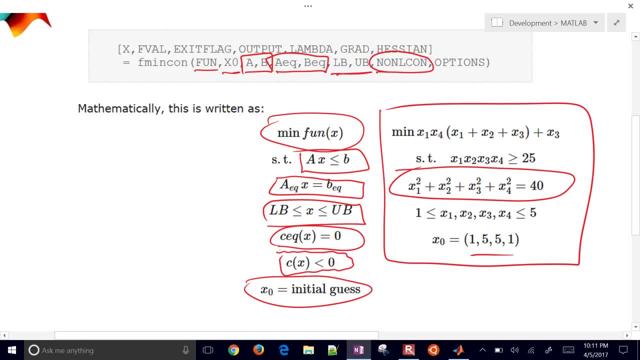 there. And then we also have our inequality constraint right here, this little st that just means subject to, so it's subject to those constraints. we also have our bounds right there, and our initial guess is right there. so we're gonna go and build this in MATLAB. so let's go ahead and just put this over in the corner and 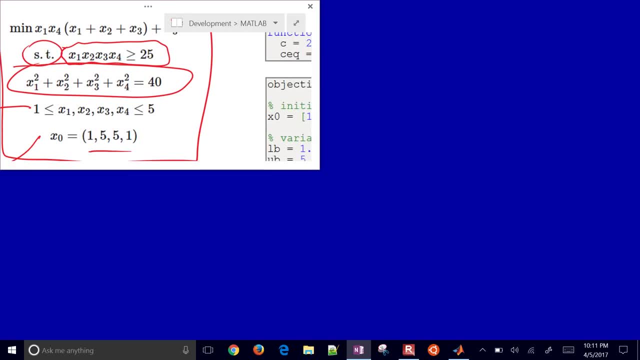 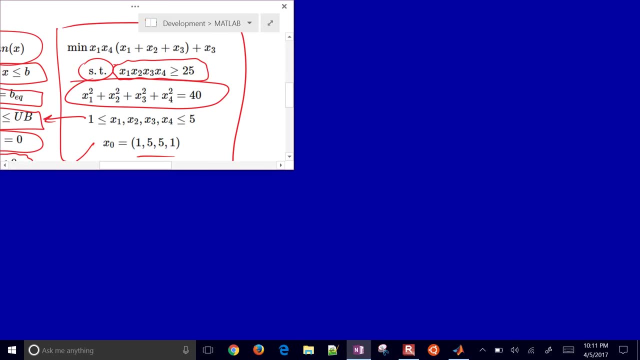 we'll go ahead and get started with this. okay, so I'll put this right here. make this just a little bit smaller. there we go and move it out of the way. all right, so there's our there. it is right there, we've got. what we want to do now is go ahead and just open up MATLAB. make sure. 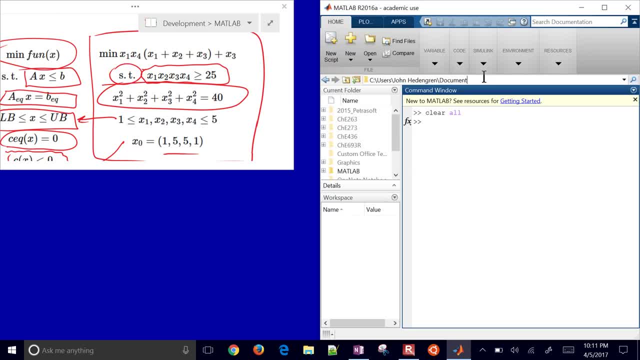 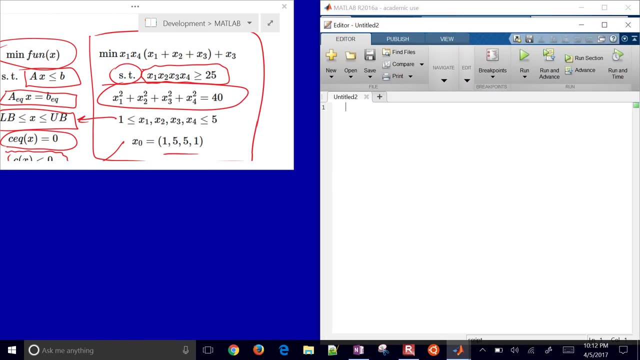 you're in the right directory, so I'm just gonna shift over to the desktop. I'll just put everything on the desktop and the first thing that we want to do is: couldn't create a new script, so we need to get a new script. okay, and do our nonlinear constraints first of. 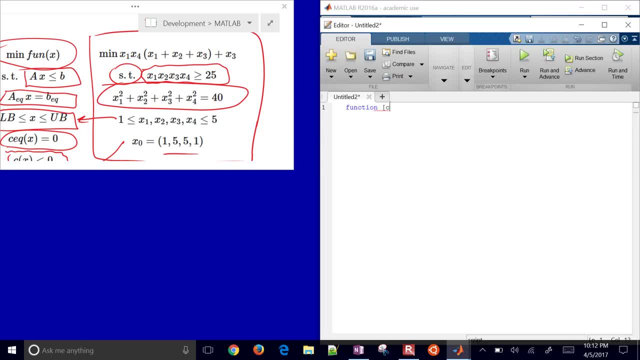 all. so I'm gonna go to create a function and I do C and C quality and I'm just gonna call this NL con and make that a function of X. okay, my very first one is gonna be my 25, and then I have to put everything on one side. 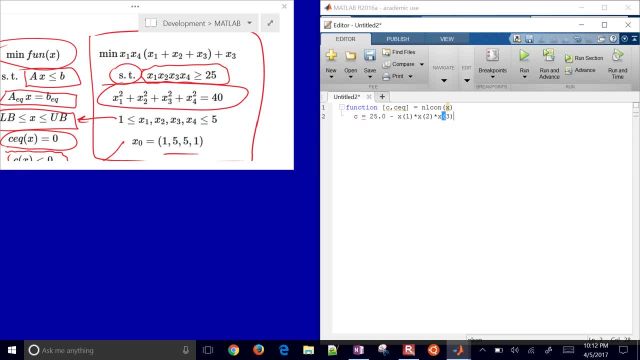 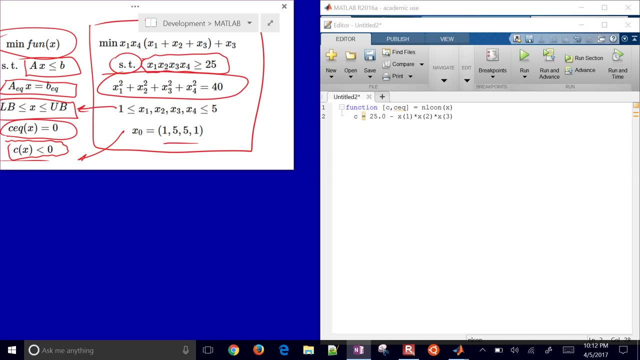 and then I have to put everything on one side, and then I have to put everything on one side, okay, of this equation, just so I can say that it's less than or equal to zero, okay, so if you remember this form right here we have to do: C of X is less than. 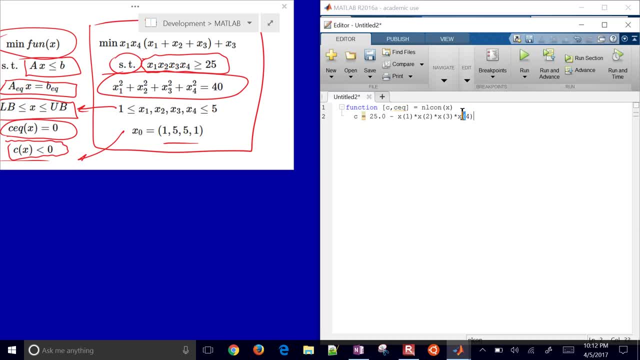 or equal to zero. I need to do also the x4 value there and so if I put that, this inequality constraint, if I move everything over it on the right-hand side and I have 25 minus, the product of all the values is less than or equal to. 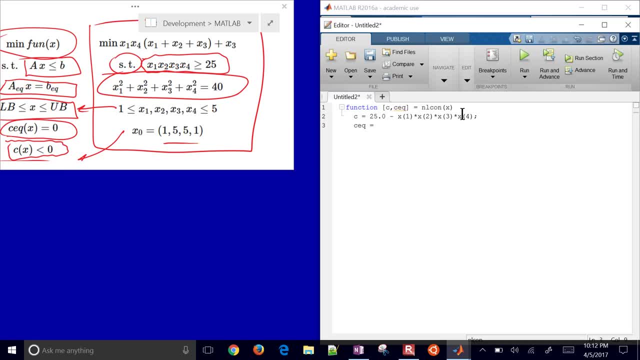 zero. okay, my equality constraint that I'm gonna do is I'm going to put it on as well. I'm going to do this in a kind of a short way with you know, operating element wise, with this dot here and then minus 40. so it doesn't matter if I do 40. 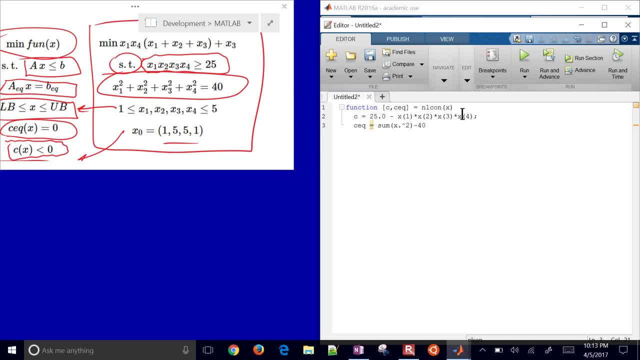 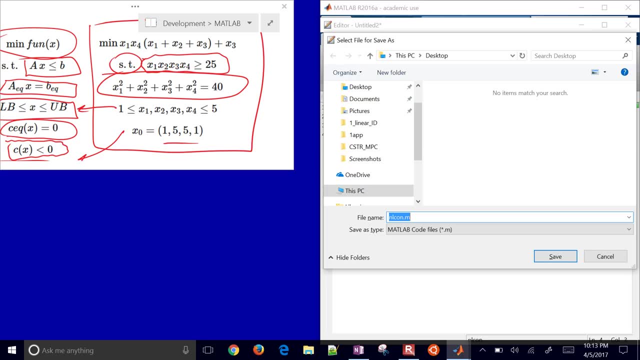 minus that sum, or sum minus that 40 equality constraints. you can put it on either side of the equation. okay, and then I go ahead and save this. it's going to suggest save it as nlconm. go ahead and click Save and then you can close that. 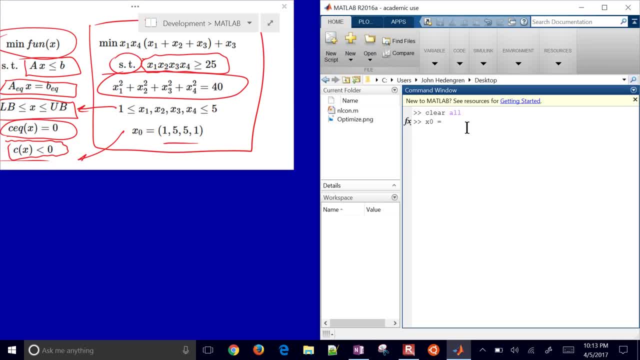 okay, let's just go and test this: my X naught. let's say I have 1, 5, 5 and 1- those are my initial values for X. and then I just want to test my C and my C equality constraints. so let's just see the residuals of those, how much they're. 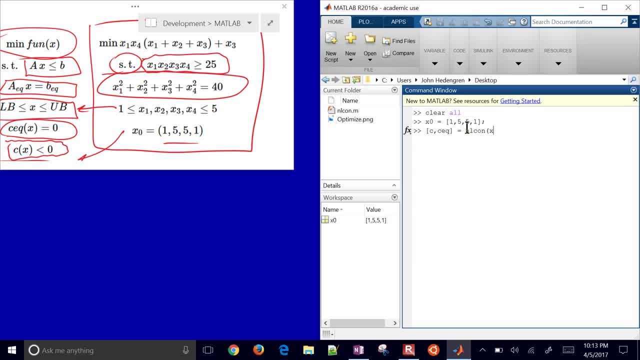 not satisfied. okay, so nlcon of X naught, and then it's going to return 0 for the very first one, so that one is exactly 0 for the very first one. so that one is exactly 0 for the very first one. so that one is exactly. 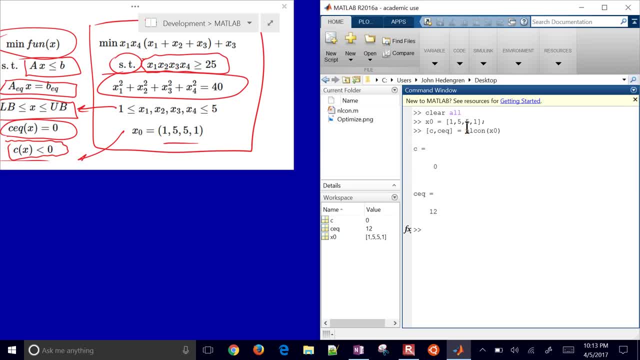 equal. so 1 times 5 times 5 times 1, that equals 25 and that is greater than or equal to 25. now, in this optimization, and when you're using continuous variables greater than or equal to or greater than their equivalent, once you get into 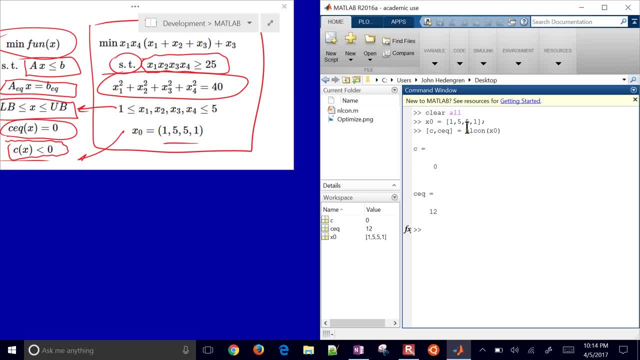 binary or integer variables, then greater than or equal to or greater than matters, but in this case those are equivalent. so those are satisfied there. okay, so we've got our nonlinear constraint first of all, got our nonlinear constraint first of all, got our nonlinear constraint first of all. now let's go ahead and just make a new. 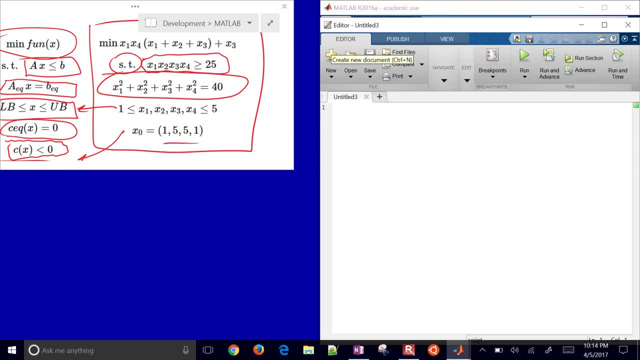 now let's go ahead and just make a new. now let's go ahead and just make a new script. okay, so, one more new script, now script. okay, so, one more new script, now script. okay, so, one more new script now. this one's gonna be our, we're gonna put. 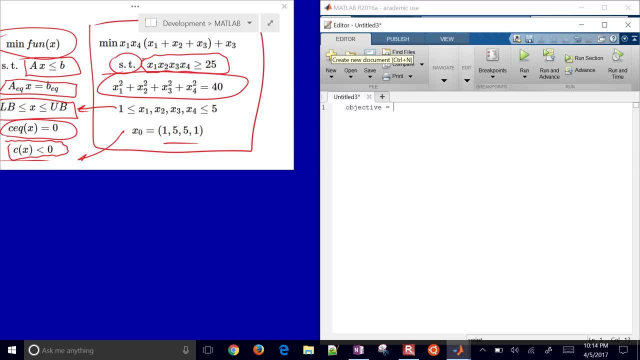 this one's gonna be our. we're gonna put this one's gonna be our. we're gonna put everything else for solving this. I'm everything else for solving this. I'm everything else for solving this. I'm gonna create. my objective is just an. gonna create. my objective is just an. 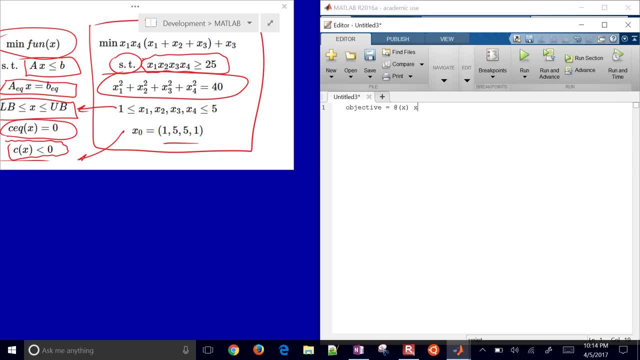 gonna create. my objective is just an inline function- anonymous function and inline function- anonymous function and inline function- anonymous function. and that one's going to be x 1 times x 4. that one's going to be x 1 times x 4. that one's going to be x 1 times x, 4 times quantity x 1. okay, and then plus x 2. 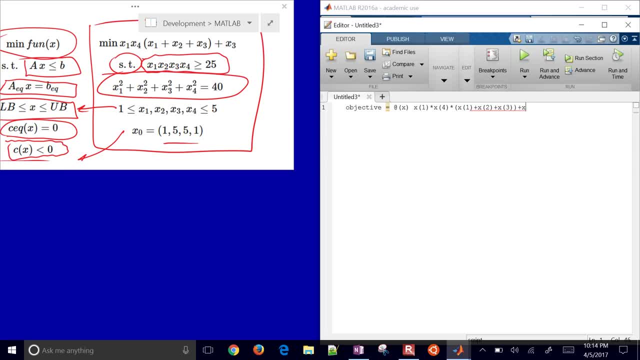 times quantity x 1- okay. and then plus x 2 times quantity x 1- okay. and then plus x 2, plus x 3- okay. plus x 3- okay. and now we plus x 3- okay, plus x 3, okay. and now we plus x 3- okay. plus x 3- okay. and now we have our objective function and let's go. 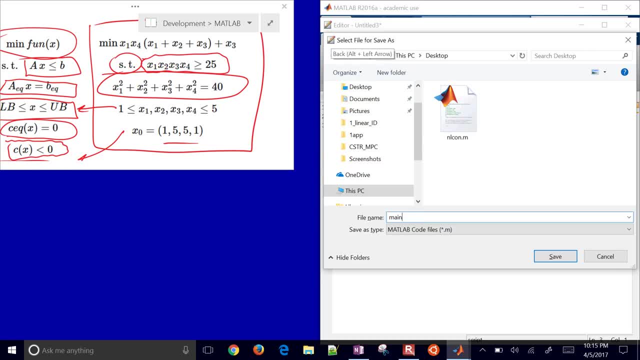 have our objective function, and let's go have our objective function and let's go ahead and save this as our- you know this- ahead and save this as our you know this ahead and save this as our you know. this is our main script that we're gonna run. 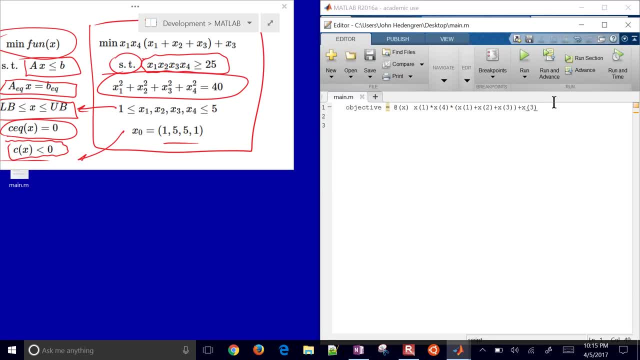 is our main script that we're gonna run, is our main script that we're gonna run and I've just put that on my desktop and I've just put that on my desktop and I've just put that on my desktop. okay, and if we want to run this and 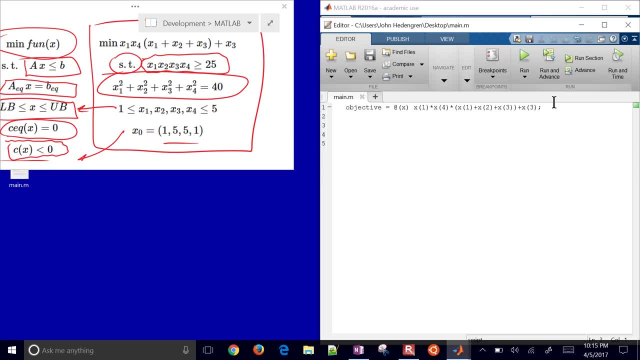 okay, and if we want to run this and okay, and if we want to run this and just test the objective function, we can just test the objective function, we can just test the objective function. we can, you know, just do objective as a function. you know, just do objective as a function. 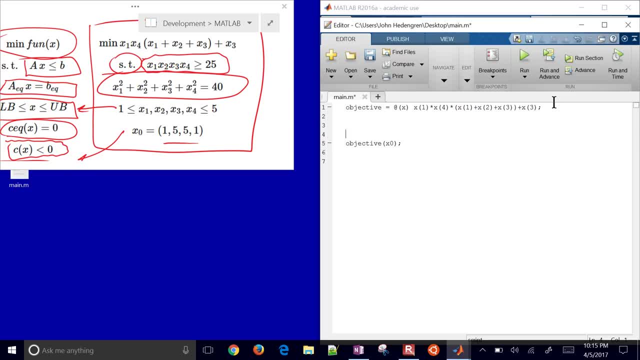 you know, just do objective as a function of X naught, and we'll do that. we'll of X naught, and we'll do that. we'll of X naught, and we'll do that. we'll return that later. okay, but let's go on. return that later, okay, but let's go on. 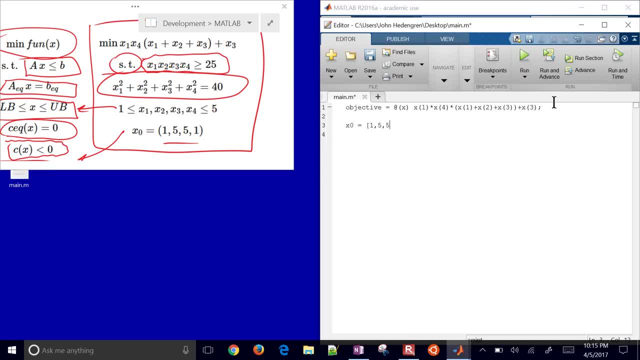 return that later. okay, but let's go on with our, just our initial guess. like we with our, just our initial guess. like we with our just our initial guess. like we had before one five, five and one: okay, had before one five, five and one- okay, had before one five, five and one: okay, there's our initial guess and then after: 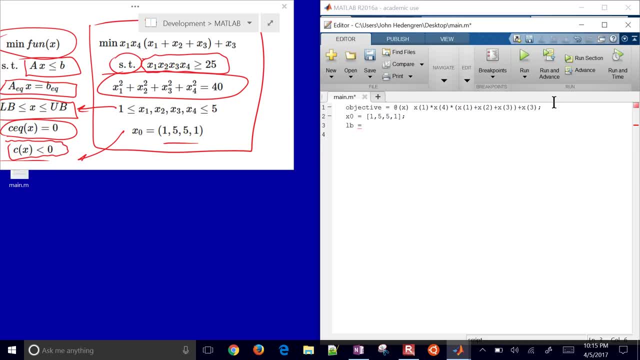 there's our initial guess, and then, after there's our initial guess, and then, after that, we're going to need to define our. that we're going to need to define our. that we're going to need to define our lower bounds. our lower bounds are going, lower bounds, our lower bounds are going. 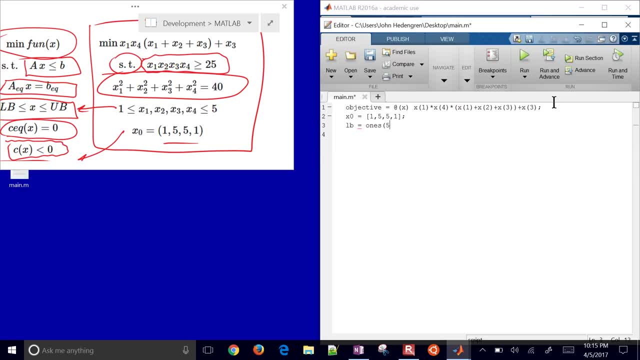 lower bounds, our lower bounds are going to be one for all of our values. so I'm to be one for all of our values. so I'm to be one for all of our values. so I'm just gonna do ones okay. a vector of just gonna do ones, okay. a vector of. 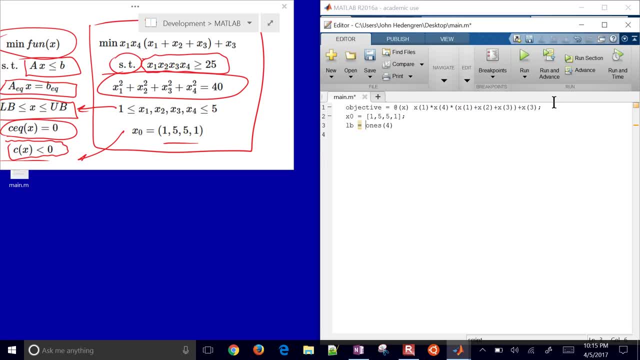 just gonna do ones okay, a vector of length four, and that's going to be times length four, and that's going to be times length four, and that's going to be times. one okay, so I've got all my ones there. one okay, so I've got all my ones there. 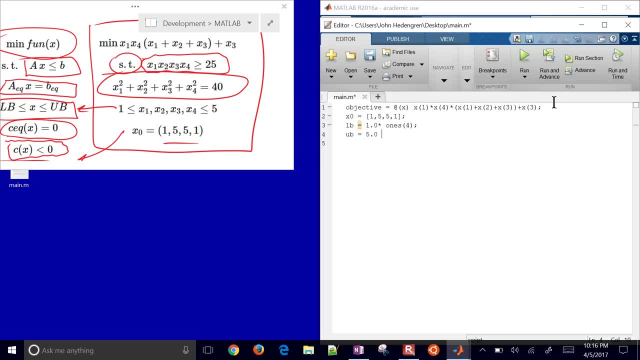 one, okay, so I've got all my ones there. and then upper bound is gonna be five, and then upper bound is gonna be five, and then upper bound is gonna be five times ones, alright. and then let's go times ones, alright. and then let's go times ones, alright. and then let's go and just display our initial objective. 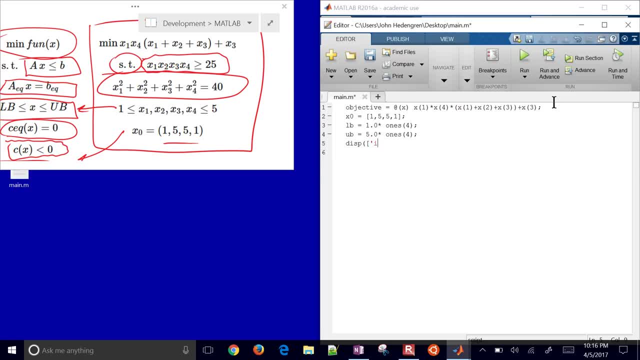 okay, and I'm gonna go ahead and put the okay, and I'm gonna go ahead and put the okay and I'm gonna go ahead and put the objective there to initial objective and objective there to initial objective and objective there to initial objective. and then, if you add in here, we're gonna do. 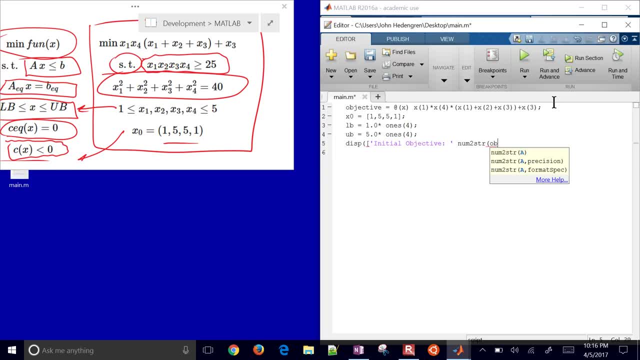 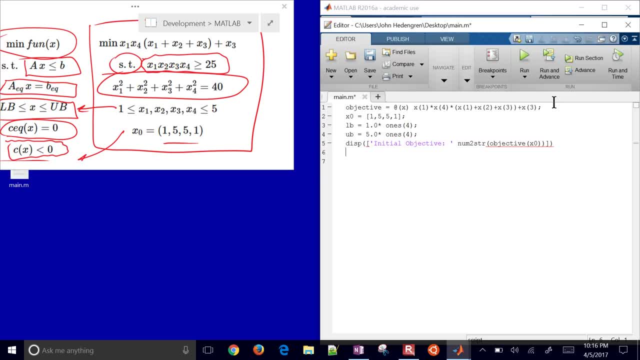 do our objective as a function of X. not okay, so there's our initial objective of X, not okay. so there's our initial objective of X, not okay. so there's our initial objective, and let's go ahead and just run, and let's go ahead and just run. 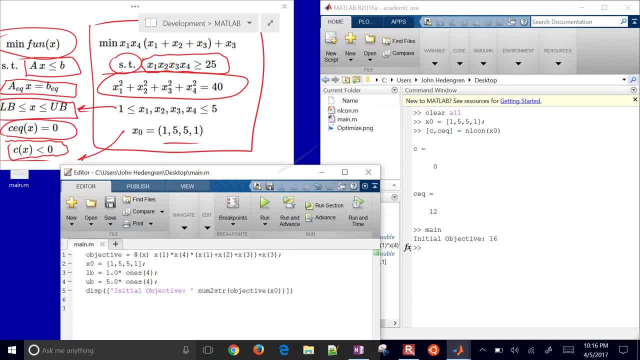 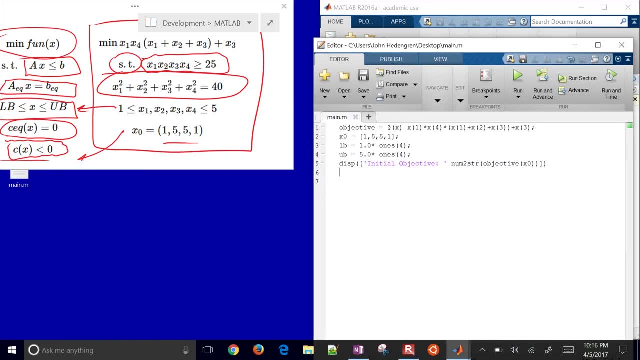 and let's go ahead and just run this, okay, and then you can see the initial: this okay. and then you can see the initial: this: okay. and then you can see the initial objective is 16. okay so, but our objective is 16. okay so, but our 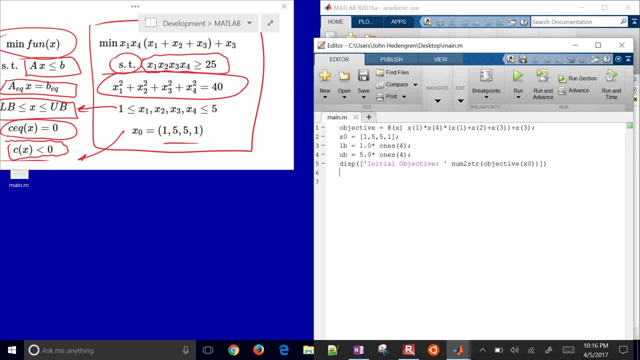 objective is 16. okay so, but our quality constraints weren't satisfied, so quality constraints weren't satisfied, so quality constraints weren't satisfied. so it might get worse than this. okay, let's, it might get worse than this. okay, let's it might get worse than this. okay, let's go on, go ahead and go on. 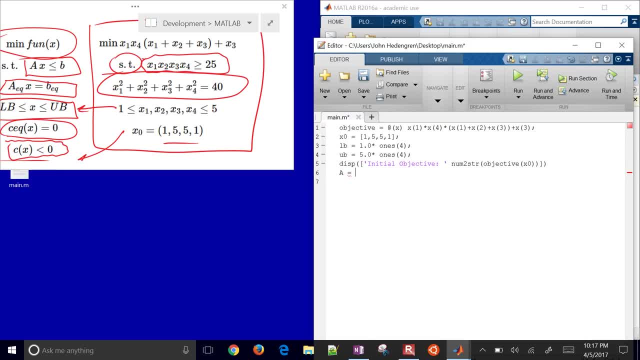 go ahead and go on, go ahead and go on. I just need to find my a value now this. I just need to find my a value now this. I just need to find my a value now. this was from you know, I just have to put in. was from you know, I just have to put in. 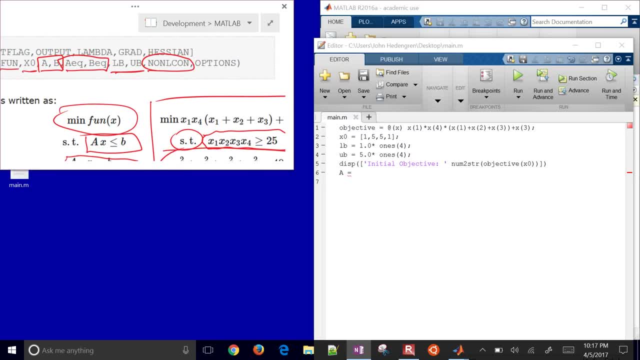 was from. you know, I just have to put in a B, a quality, B quality, and those are a B, a quality, B quality, and those are a B, a quality, B quality, and those are just gonna be empty. okay, so what, I'm just gonna be empty. okay, so what I'm. 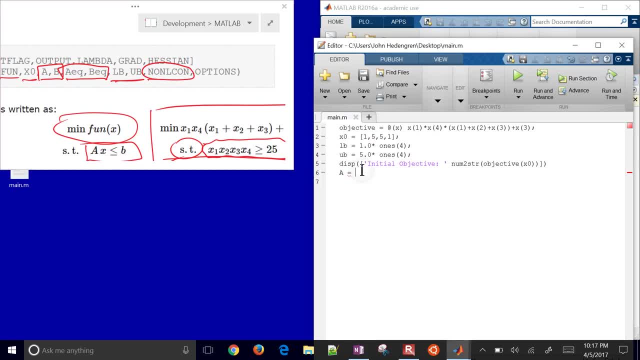 just gonna be empty, okay. so what I'm gonna do here is is just couldn't put in. gonna do here is: is just couldn't put in. gonna do here is: is just couldn't put in an empty array- okay, a, B, empty, a quality. an empty array, okay, a, B, empty, a quality. 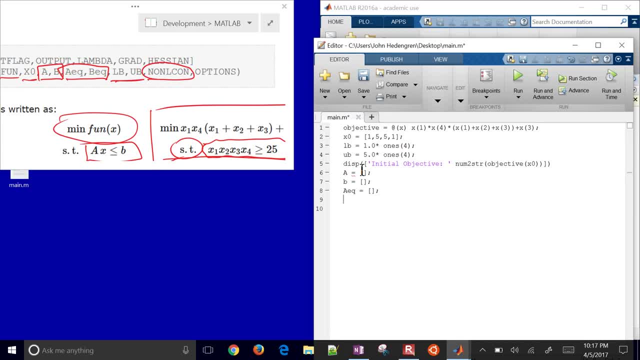 an empty array, okay, a, B empty. a quality is going to be empty as well, is going to be empty as well, is going to be empty as well. and B quality empty as well. so if you and B quality empty as well, so if you and B quality empty as well. so if you have linear equations, you put those in. 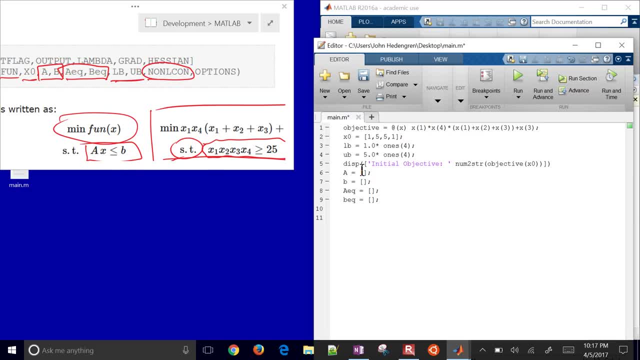 have linear equations, you put those in. have linear equations, you put those in there. but for this case we don't have there. but for this case we don't have there, but for this case we don't have any linear equations. okay, let's go on to any linear equations. okay, let's go on to. 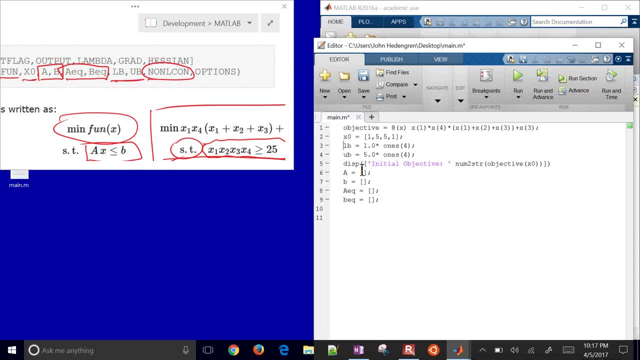 any linear equations. okay, let's go on to our we have lower and upper bounds. our we have lower and upper bounds. our we have lower and upper bounds. we're gonna put those in the order in. we're gonna put those in the order in. we're gonna put those in the order in which you have to display them to find. 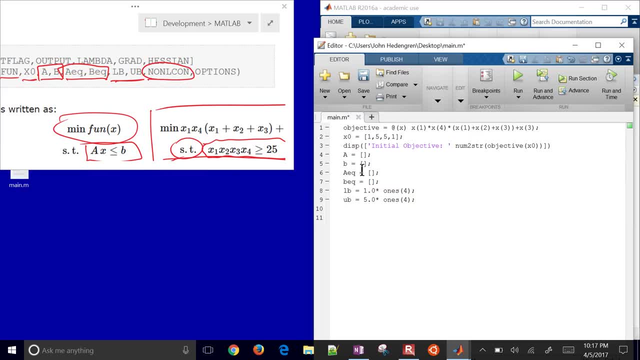 which you have to display them to find, which you have to display them to find them. okay, and we don't have to define them. okay, and we don't have to define them okay, and we don't have to define them in any order, but just the way they. 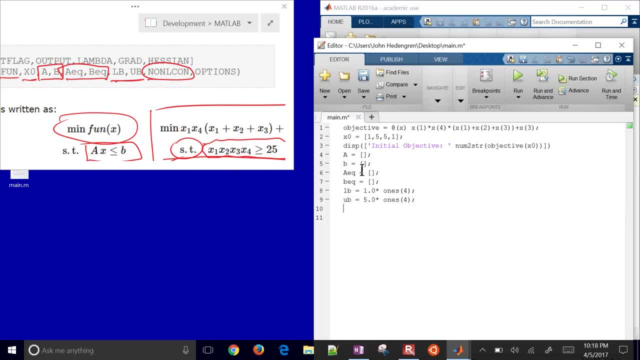 them in any order, but just the way they them in any order, but just the way they appear in the F min con function and appear in the F min con function and appear in the F min con function, and then we also need to give a function. then we also need to give a function. 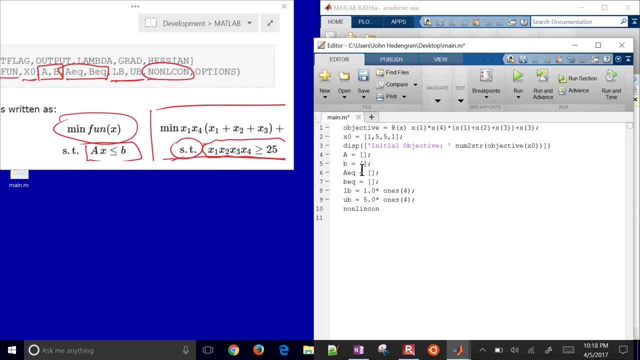 then we also need to give a function: handle, okay, you can. you can name this. handle, okay, you can. you can name this. handle okay, you can. you can name this whatever you want. I'm just gonna name whatever you want. I'm just gonna name whatever you want. I'm just gonna name this and L? con equals the at sign and L. 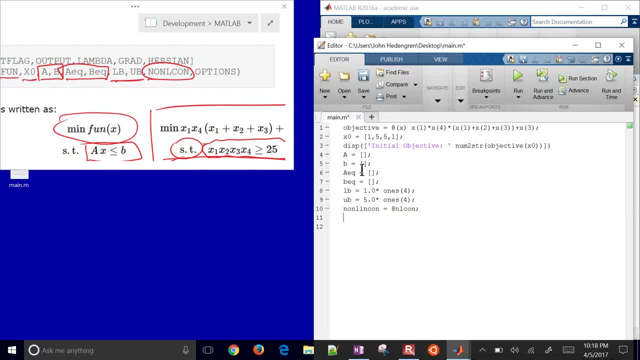 this and L con equals the at sign and L this and L con equals the at sign and L con. and there we have all of our con and there we have all of our con, and there we have all of our options that we need. now we can use F. 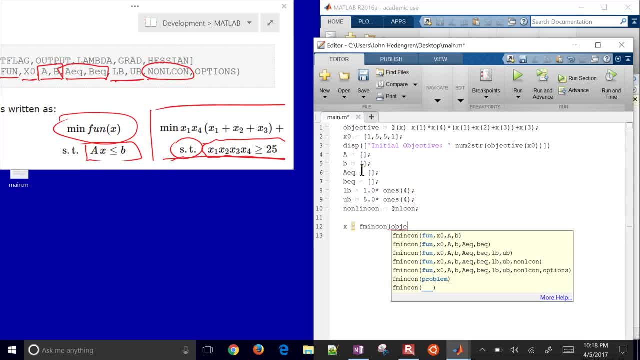 options that we need now. we can use F options that we need now. we can use F min con to solve this. so we have our min con to solve this. so we have our min con to solve this. so we have our objective. we have X naught and we have a. 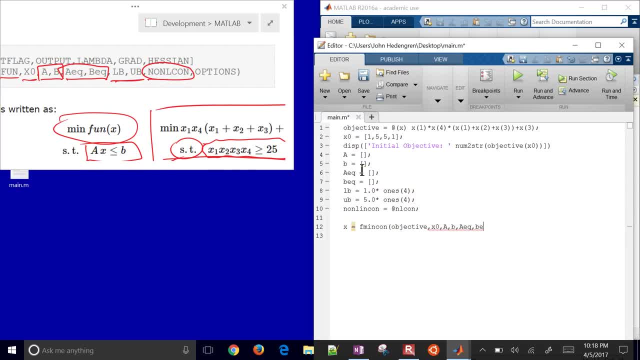 objective. we have X naught and we have a objective. we have X naught and we have a and B and a quality and B quality, and and B and a quality and B quality, and and B and a quality and B quality, and our lower bound, upper bounds and our 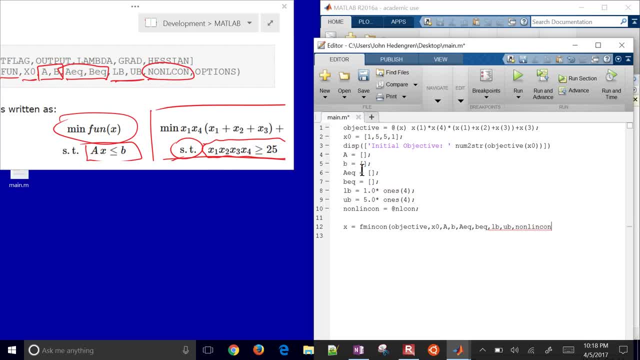 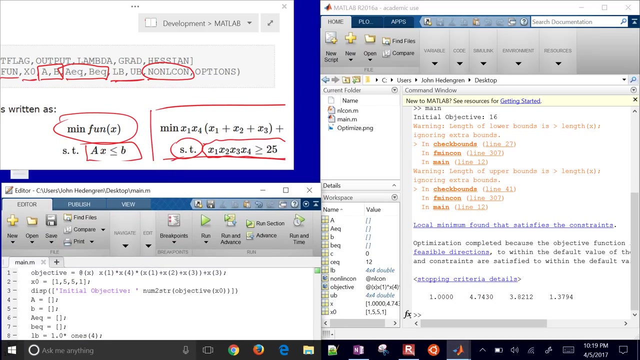 our lower bound upper bounds and our, our lower bound upper bounds and our non-linear constraint, non-linear constraint, non-linear constraint, okay, okay, okay, and let's go ahead and do this, and, and let's go ahead and do this, and and let's go ahead and do this, and let's go ahead and test what our final. 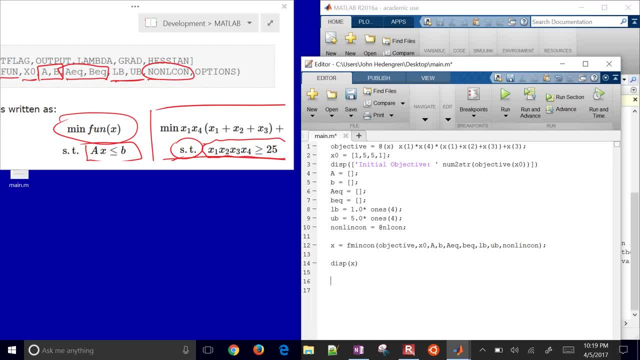 let's go ahead and test what our final, let's go ahead and test what our final objective is as well. so either you can- objective is as well, so either you can, objective is as well. so either you can do you know, create another output, or you do you know create another output, or you. 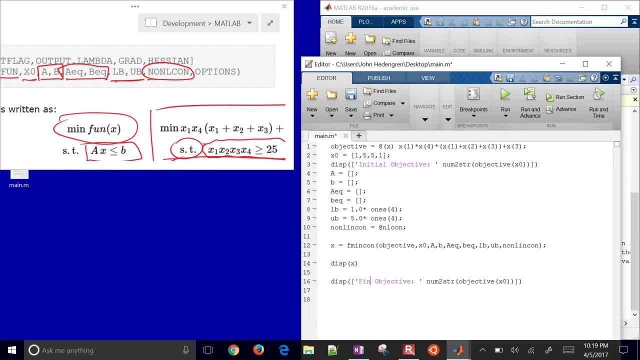 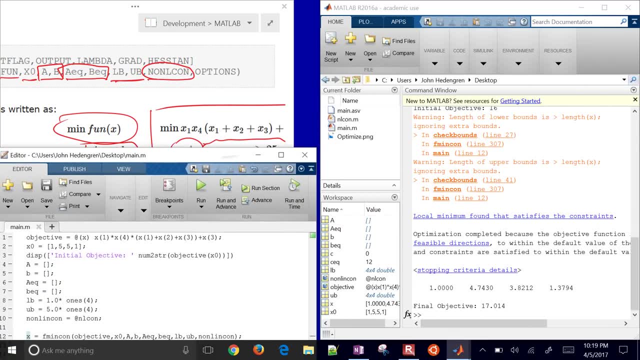 do you know, create another output. or you can also just say final objective plug, can also just say final objective plug, can also just say final objective, plug that back in. and let's go ahead and plug that back in. and let's go ahead and plug that back in. and let's go ahead and plug in X instead of X, naught, and then it. 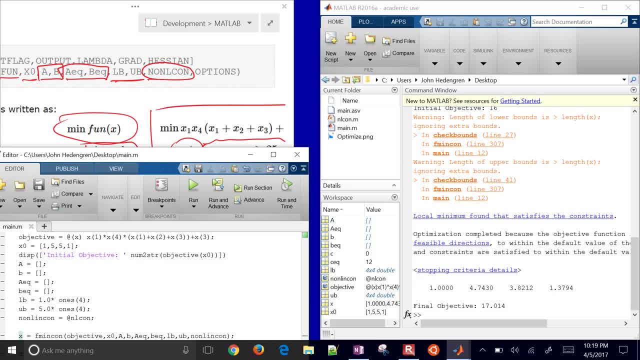 in X instead of X naught, and then it in X instead of X naught, and then it will show you your final objective, as will show you your final objective, as will show you your final objective as well. now, you see, it got worse than 16. 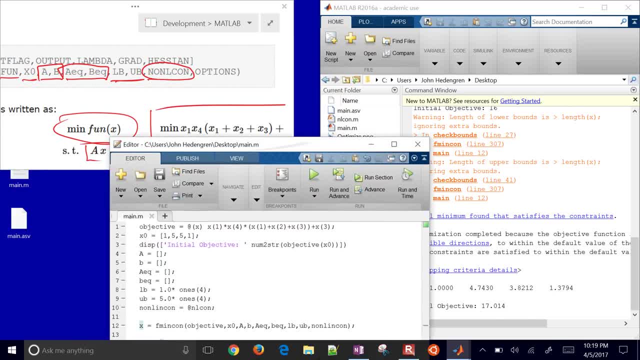 well, now you see it got worse than 16. well, now you see it got worse than 16. but in this case, let's go and check and. but in this case, let's go and check and. but in this case, let's go and check and see if it satisfied our constraints. okay, 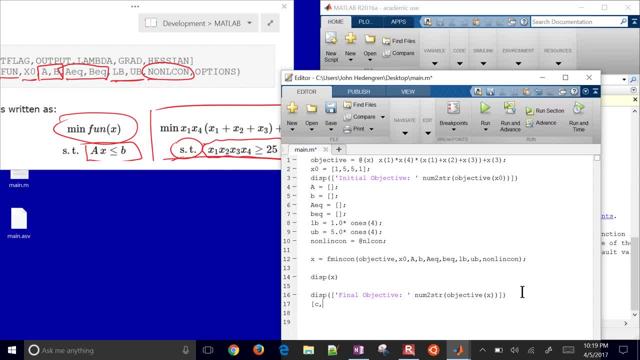 see if it satisfied our constraints, okay. see if it satisfied our constraints, okay. and if you want to just do that, you can, and if you want to just do that, you can, and if you want to just do that, you can do. a CC quality equals NL con as a. 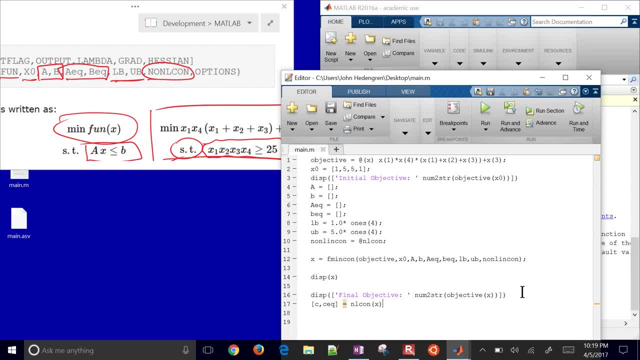 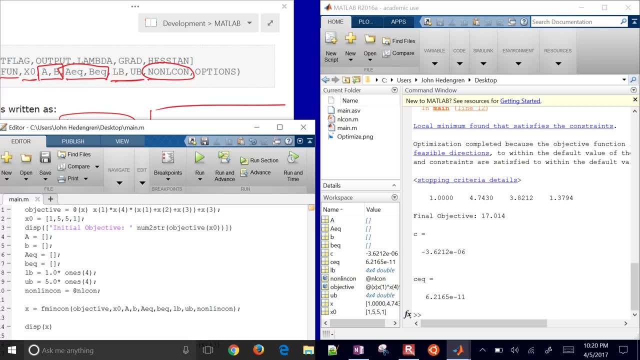 do a CC quality equals NL con as a. do a CC quality equals NL con as a function of X and run that one more time. function of X and run that one more time. function of X and run that one more time. okay, so you can see that the inequality. 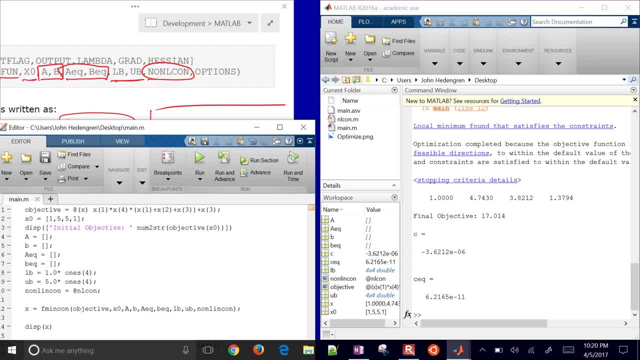 okay, so you can see that the inequality. okay, so you can see that the inequality: it's less than zero. you can see it's, it's less than zero. you can see it's it's less than zero. you can see it's negative three times e to the 10, to the. 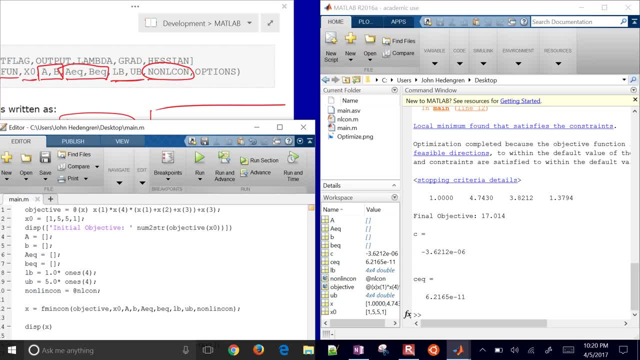 negative three times e to the 10 to the negative three times e to the 10 to the minus six, okay, and then you also have minus six, okay, and then you also have minus six, okay, and then you also have equality constraint. that's nearly equal. equality constraint, that's nearly equal. 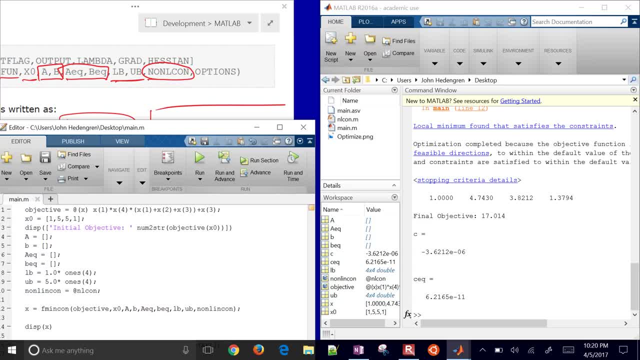 equality constraint that's nearly equal to zero. but an optimization there to zero. but an optimization there to zero, but an optimization there. convergence tolerances that say as long. convergence tolerances that say as long. convergence tolerances that say as long as you're within a certain amount of. 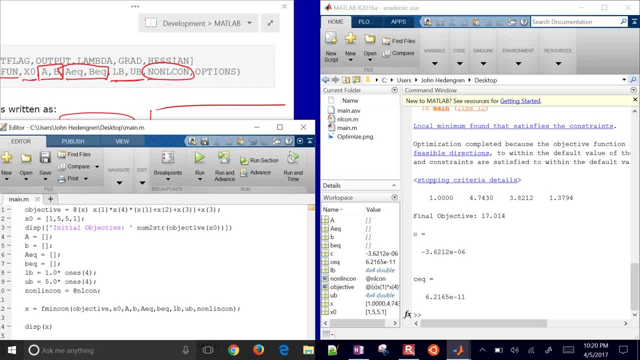 as you're within a certain amount of, as you're within a certain amount of that constraint, then you're okay. okay, so that constraint, then you're okay. okay, so that constraint, then you're okay, okay. so there we have it, the quality, and there we have it, the quality, and 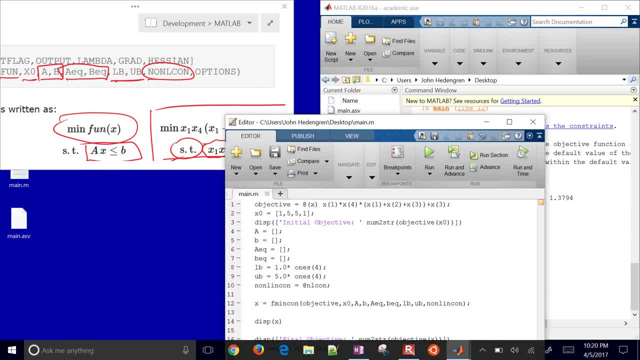 there we have it. the quality and inequality constraints are satisfied now. inequality constraints are satisfied now. inequality constraints are satisfied now. you can also have other things that are. you can also have other things that are. you can also have other things that are. come back from F min con if you didn't. 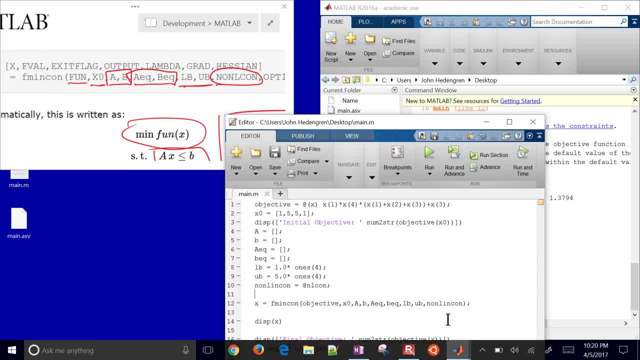 come back from F min con, if you didn't come back from F min con, if you didn't want to have to evaluate that objective, want to have to evaluate that objective, want to have to evaluate that objective, function that final objective you can. function that final objective you can. 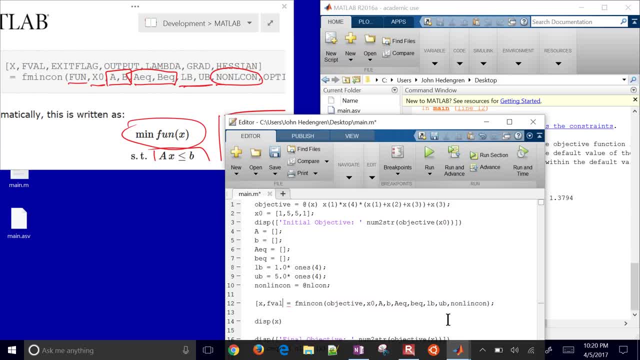 function, that final objective. you can also say that X and then FL and exit. also say that X and then FL and exit. also say that X and then FL and exit. flag and I'll do an output there you can. flag and I'll do an output there you can. 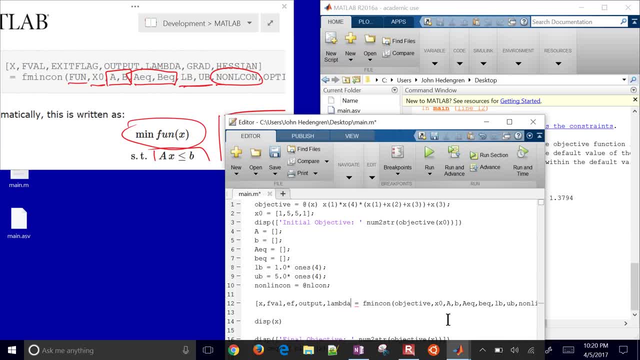 flag and I'll do an output there. you can also get your Lagrange multipliers lambda. also get your Lagrange multipliers lambda. also get your Lagrange multipliers lambda and your gradients and your Hessians and your gradients and your Hessians and your gradients and your Hessians, if you want. okay, so let's go ahead and run. 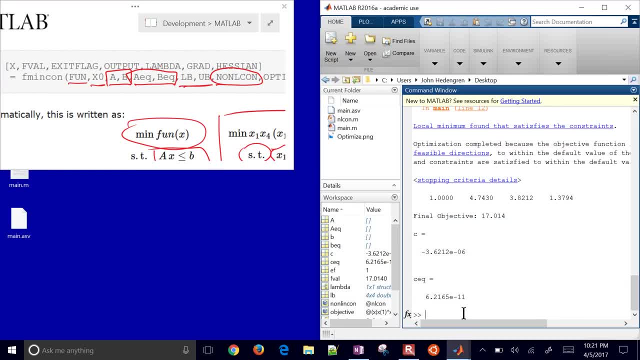 if you want, okay, so let's go ahead and run. if you want, okay, so let's go ahead and run that one more time. okay, so we got a that one more time. okay. so we got a that one more time. okay. so we got a bunch of stuff here let's look at for. 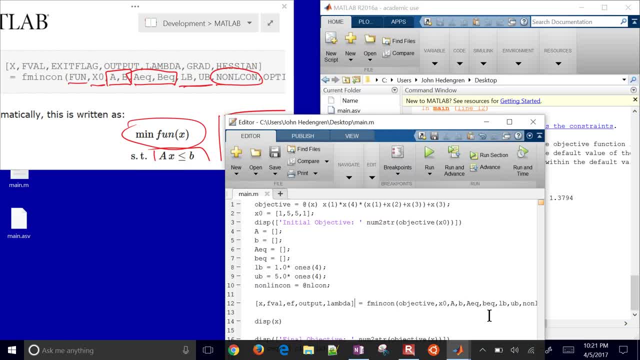 bunch of stuff here. let's look at for bunch of stuff here. let's look at, for example, our okay, our FL there you had example. our okay, our FL there, you had example. our okay, our FL. there you had the. the objective- this report is optimal. the- the objective: this report is optimal. 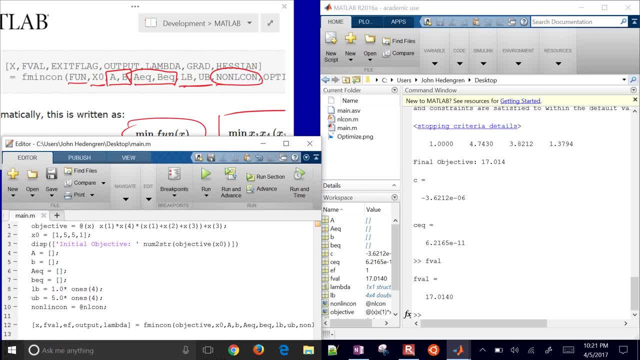 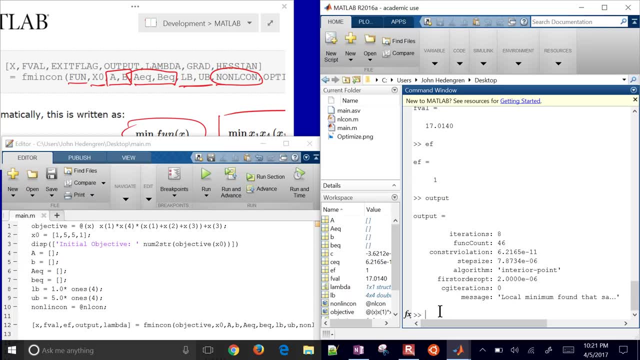 the the objective. this report is optimal. you also have. you know some other things. you also have. you know some other things. you also have you know some other things in there as well. you have the exit flag in there as well. you have the exit flag in there as well. you have the exit flag. okay, that means success. and then you 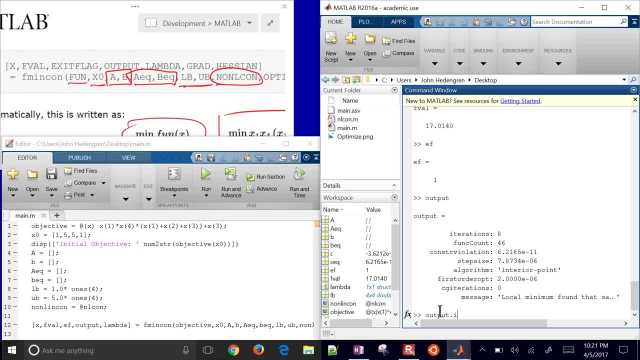 okay, that means success. and then you: okay, that means success, and then you also have your output there. you can see, also have your output there. you can see, also have your output there. you can see output iterations. okay, you can just output iterations. okay, you can just output iterations. okay, you can just display that. if you want, you have. 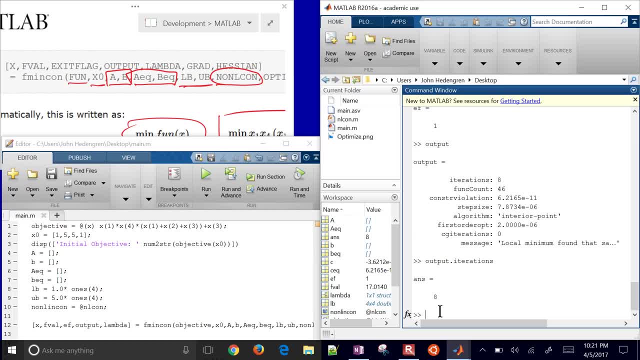 display that. if you want, you have display that. if you want, you have function count. you have constraint function count. you have constraint function count. you have constraint violation, step size. all these other violation, step size, all these other violation, step size, all these other algorithm options and and things that. 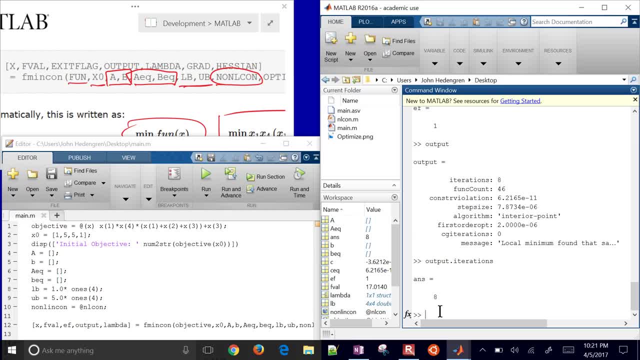 algorithm, options and and things that were used for solving the problem- okay. were used for solving the problem- okay. were used for solving the problem, okay. so it found a local minimum. okay, and so it found a local minimum. okay, and so it found a local minimum. okay. and then lambda- let's go and print lambda. 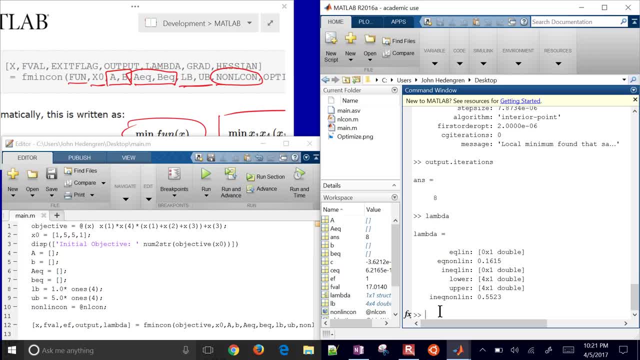 then lambda- let's go and print lambda. then lambda- let's go and print lambda. is our Lagrange multipliers comes back? is our Lagrange multipliers comes back? is our Lagrange multipliers comes back as a structure? so you have to print the as a structure. so you have to print the. 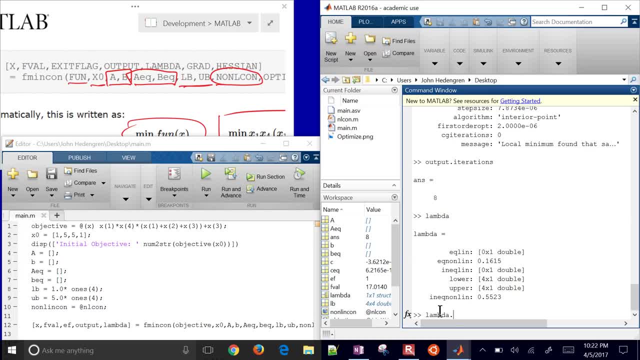 as a structure. so you have to print the one that you want, okay. and let's say we one that you want, okay. and let's say we one that you want okay. and let's say: we want our inequality equation for a. want our inequality equation for a. 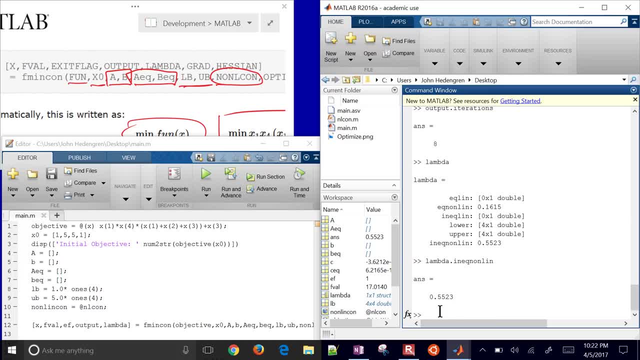 want our inequality equation for a? nonlinear- okay there, it is nonlinear. okay there, it is nonlinear. okay there, it is right there. okay, so we had a. we had our right there. okay, so we had a. we had our right there. okay, so we had a. we had our equality nonlinear constraint, Lagrange. 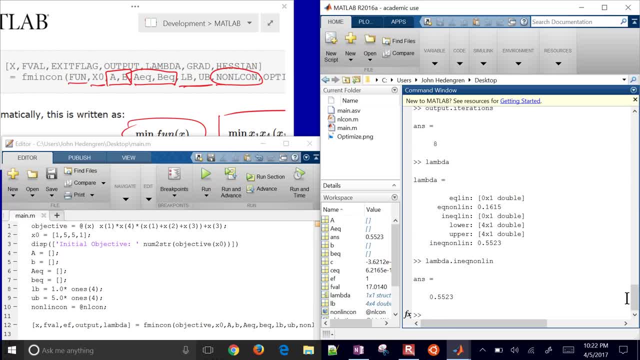 equality- nonlinear constraint- Lagrange equality- nonlinear constraint- Lagrange multiplier- now I can't play risk okay, multiplier. now I can't play risk okay, multiplier. now I can't play risk okay. and let's, let's okay, so this is our, and let's, let's okay, so this is our. 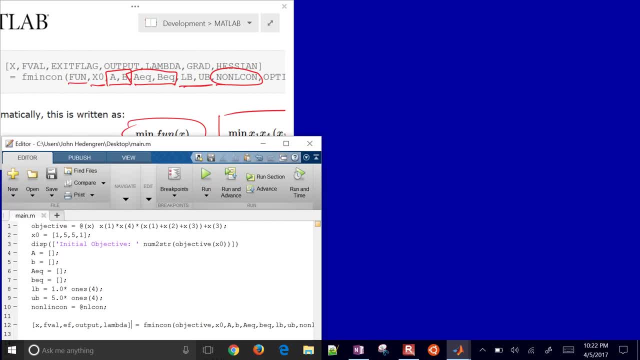 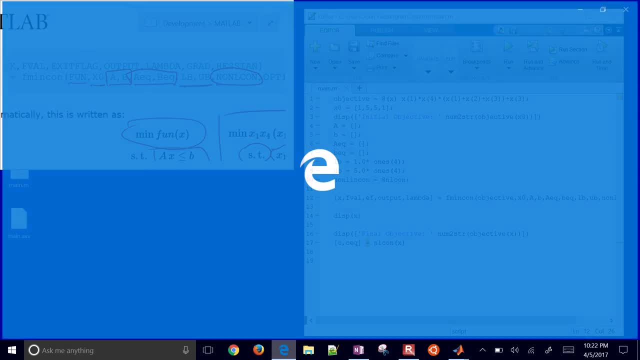 and let's, let's, okay, so this is our optimization problem. right here, we've optimization problem. right here, we've optimization problem. right here, we've solved it with F min con and okay, that's solved it with F min con. and okay, that's solved it with F min con and okay, that's it again. if you want to download the,